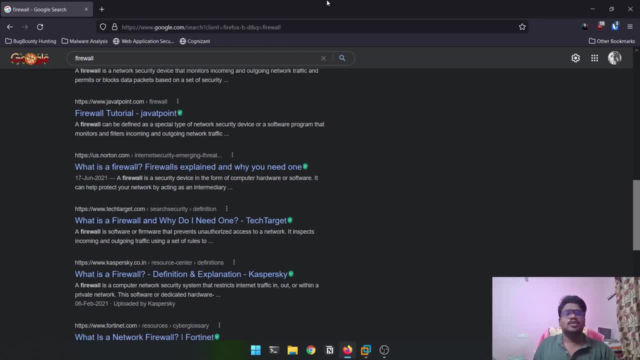 okay, so he monitors everything, everything. so if you consider a web application, so most of the publications out there on internet or some top companies, uh, always use some kind of a firewall. so the reason why they use firewall is like, like, whenever we are trying to do some attacks, like 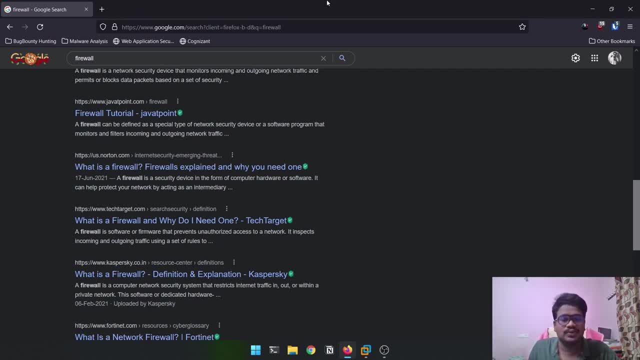 a remote command execution or os command execution or cross-site scripting payloads. so these are nothing but the payloads, right? so while sending to the payloads, uh, while sending the from our machine to that server, so this particular firewall detects those kinds of five payloads and it it filters the stuff, okay, so that is the reason. uh, it is always a better, uh, better way. 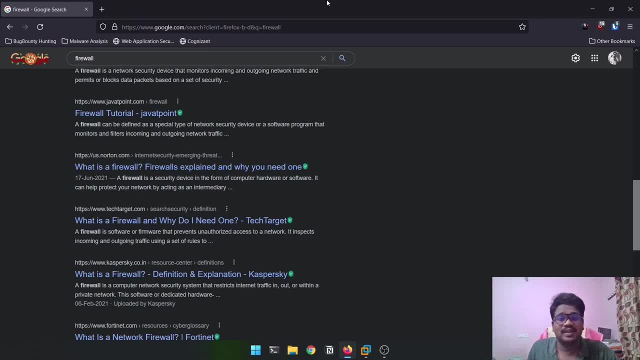 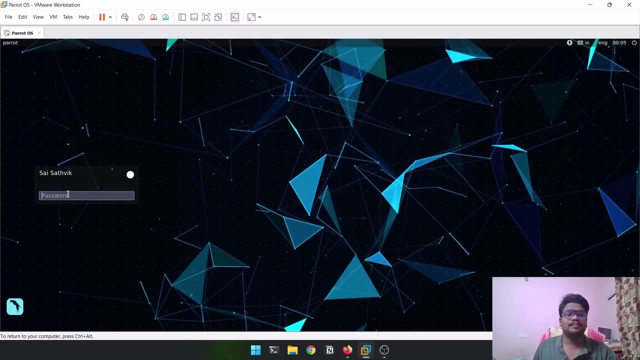 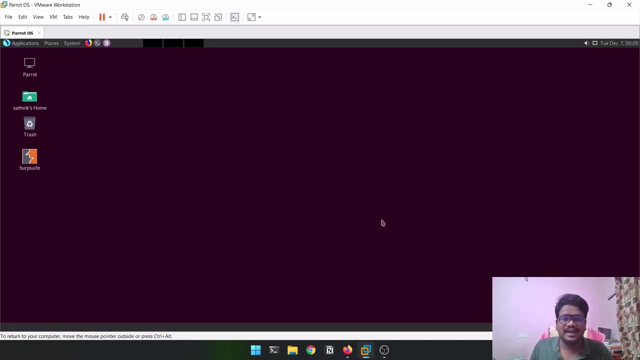 to understand what the uh, what firewall, that particular company is using. so there are some few tools uh, i'm going to showcase in this video. so let me open my uh para toys. i'm going to demonstrate this process on a parrot os and also guys. everything that i'm going to show you are not any harmful content. it. 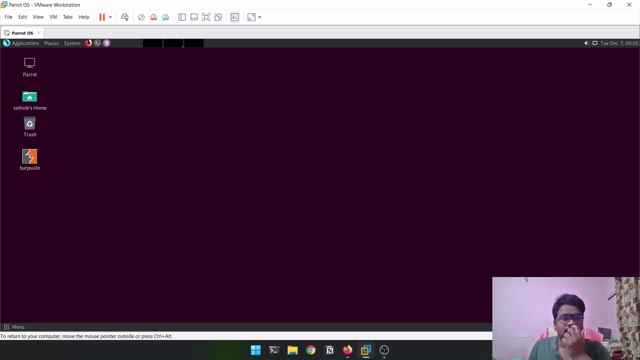 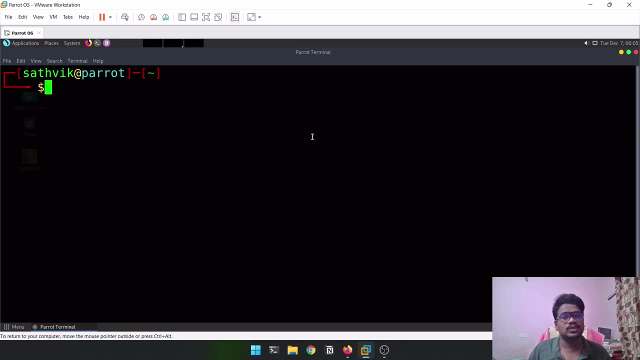 is just like an information gathering step. okay, so let me open my terminal. so the first tool that we know, or the first tool that we are going to use, is most commonly known tool, which is nothing but nmap. so yes, in nmap there is a section called as nmap scripting engine, which ends with the extension. 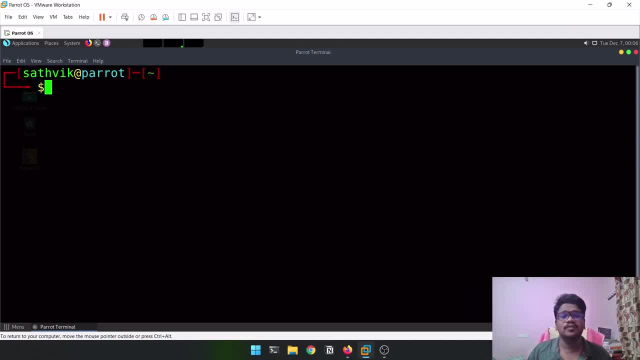 ok, there are some few scripts which we can make use of and we can do the stuff. so let me show you those scripts right now. so locate dot nsc and i'm graphing for http vaf. so vav in the sense of application firewall. so i passed a simple uh. 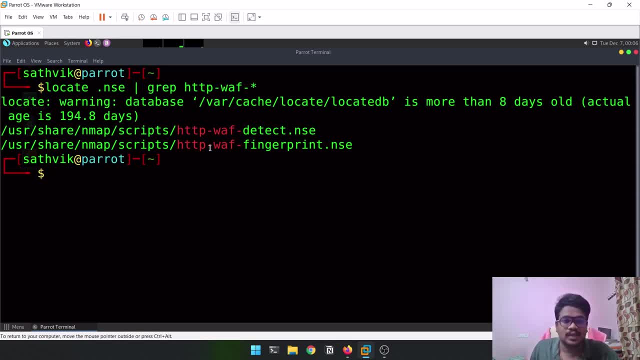 rejects kind of thing. and you can see these are some few nmap scripts so you can see uh, http hyphen detect and http-wav-fingerprint. so these are some scripts which help you in identifying the this particular firewall. i'm going to show you that just a minute. i'm going to open a new tab. 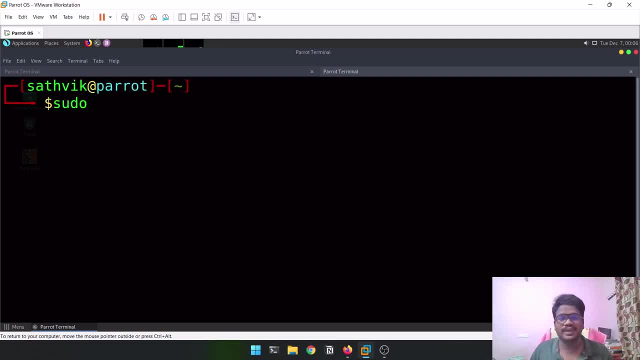 so it is simple. so sudo. the reason i'm using sudo here is because i'm not the root user on my paratois, i'm just a normal user. so nmap and i'm going to specify the port. so mostly, if you consider, as we're considering the web application firewall, so in most of the cases it will be on. 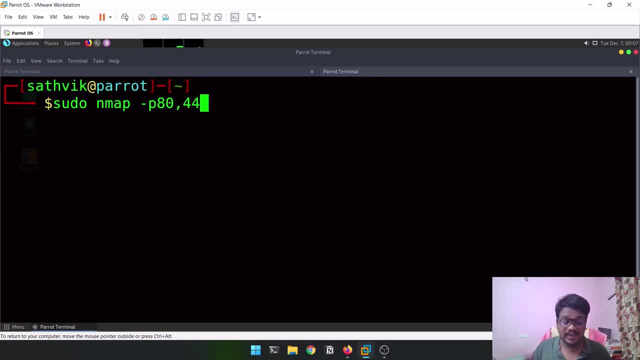 port 80 or 443, and there are few cases like there might be some server running on some different ports. like any port, a port number can be anything, so in that case you can provide those ports as well. like, let us assume that 8080 is a port available or 8080 is the port which is offering. 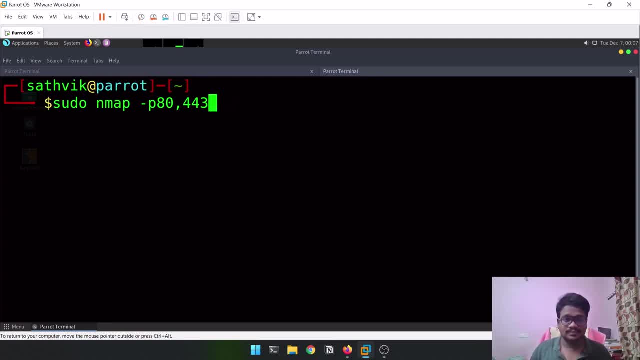 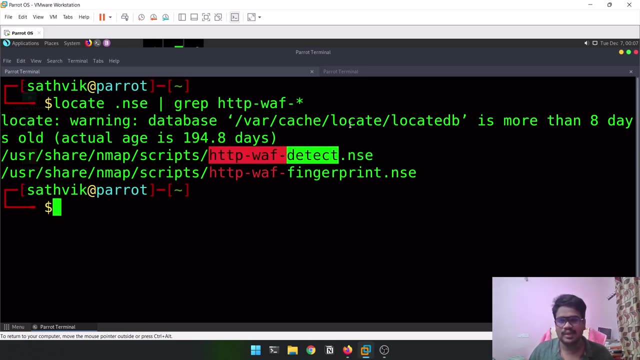 this particular web application service. you can add that, okay, and there is a parameter you need to specify, which is hyphen, hyphen script and equal to. so what you can do is like you can simply copy only this part. you don't need to provide the extension as well. extension, okay, you can simply copy that, you can paste that and 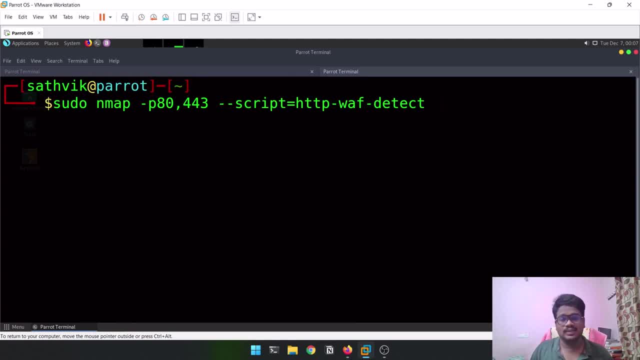 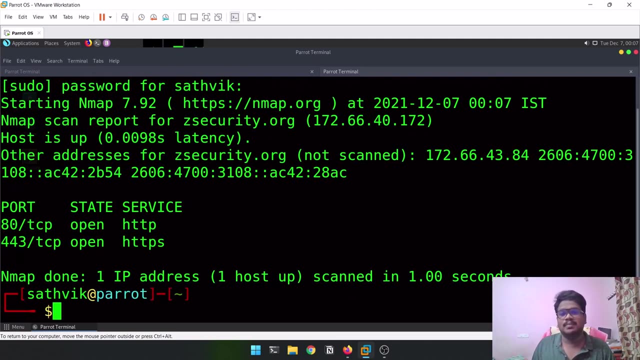 you can provide the ip address. okay, it can be anything, so i'm not going to show you anything. you can simply like you can provide the jet security dot org. as i told you, this is not any harmful thing, okay, but there is a problem with the nmap as well. i'm going 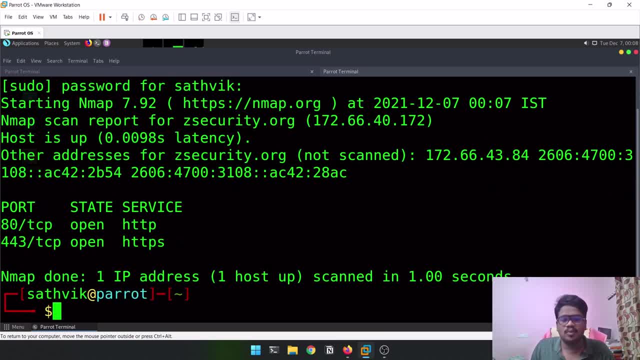 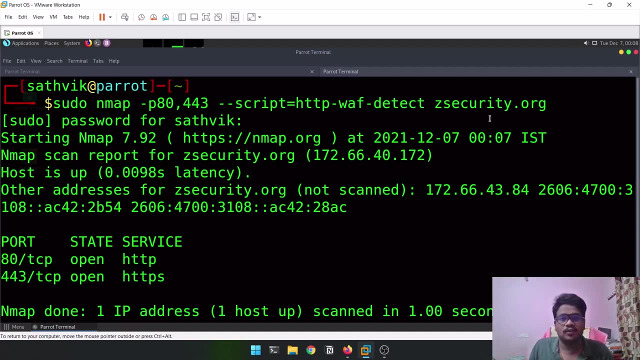 to show. i'm going to tell you that. okay, the reason is, like most of the times while i'm using this particular scripts from nmap, like it is not showing me the option out there. okay, so if you consider this, uh, jet security dot org, they have, uh, uh, what you call this cloudfare. 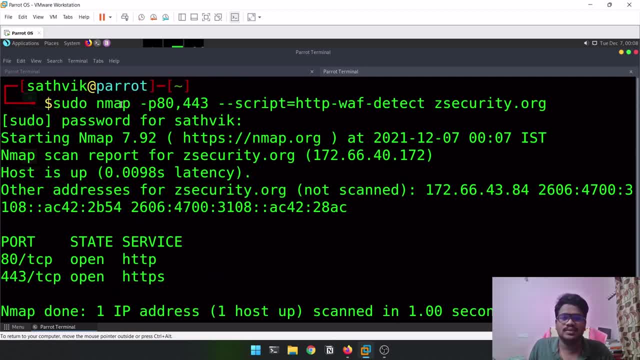 firewall okay, but most of the time, uh, when i use this nmap, uh it it haven't detected some stuff, like it is like chances like 50 percent of the times it had shown me what kind of firewall it is and most of the time it is like 50 percent of the time it haven't shown me. so it is dependent, like 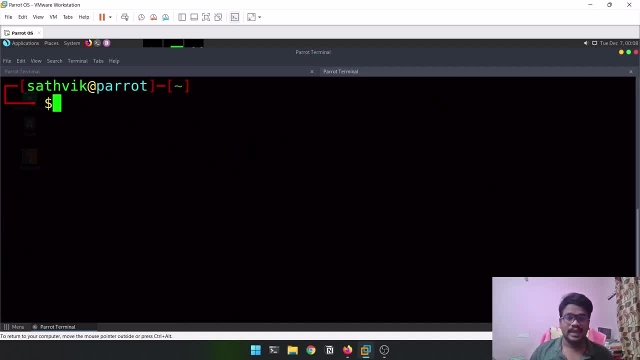 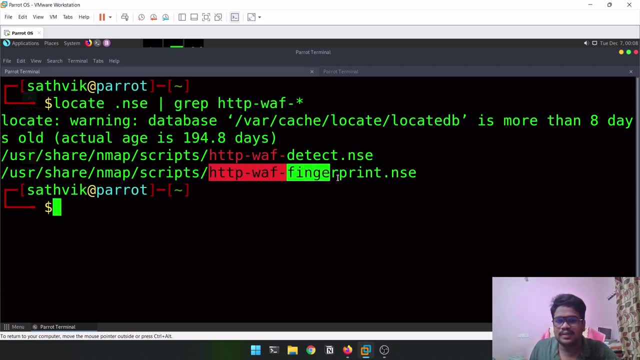 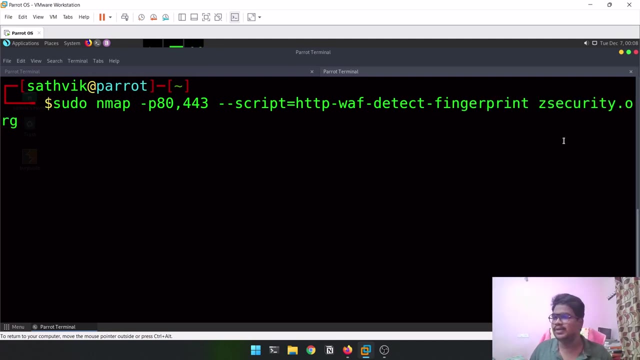 but uh, knowing what the like, knowing how to do, is always helpful to you. okay, and also, there is another script here, so we completed the usage of the script, like, uh, we can provide the script as well, fingerprint and you can try your luck. okay, and also, guys here you can provide, like i provide. 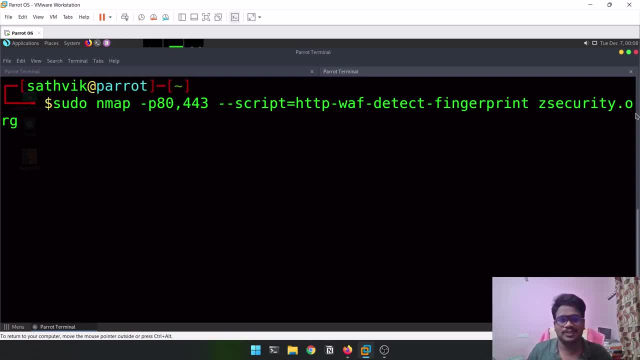 the domain name, but you can always provide an ip address, okay, of your choice. so, with with the being said, this is how you can make use of nmap scripting engine in order to detect the firewall of a web application- not only the web application, but sometimes it even detects the uh firewall on. 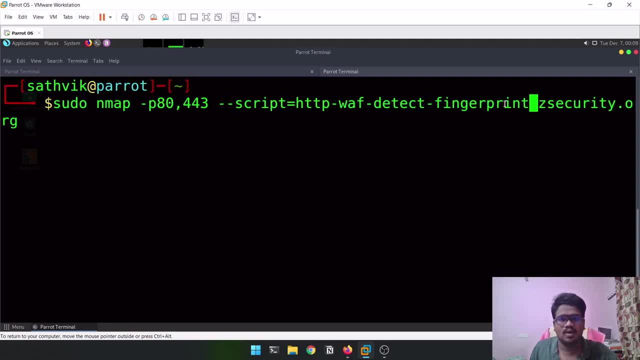 uh, ip address like normal operating systems as well, or normal machines as well, so you can make sure you make sure to check that out, okay? so, that being said, i'm going to stop this particular thing and i'm going to showcase another tool. okay, so there is a. 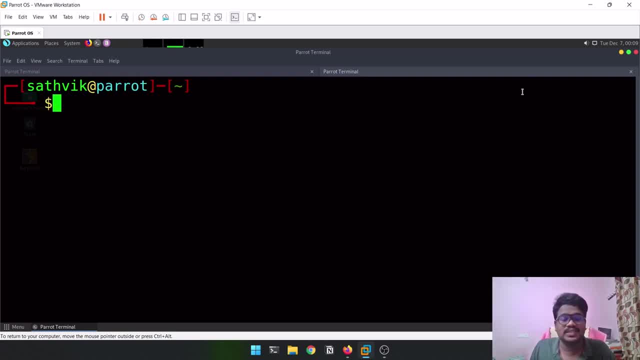 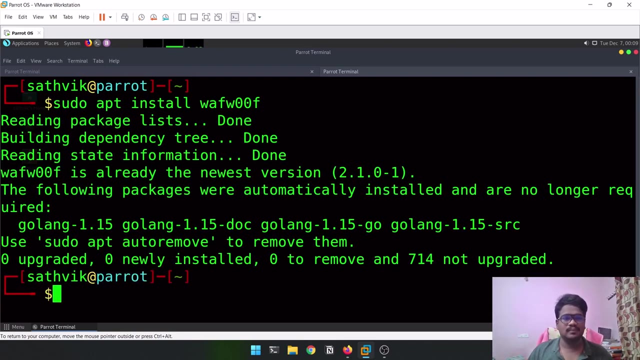 one more cool tool, like most popular tool out there, which is wav woof. so you know you need to install that thing. so sudo apt, install wav w zero, zero, it's not o move. uh, you can install. that's a simple thing, like most of the times. if you are using any hacking distribution like parrot or 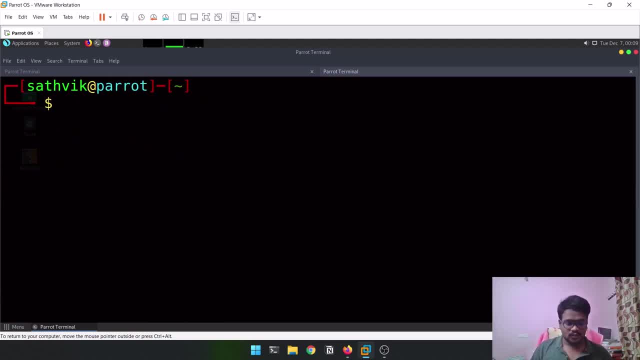 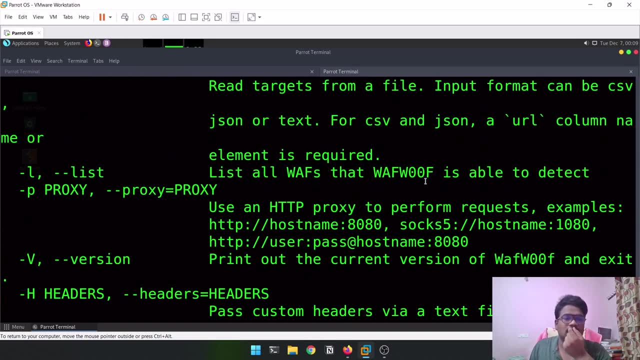 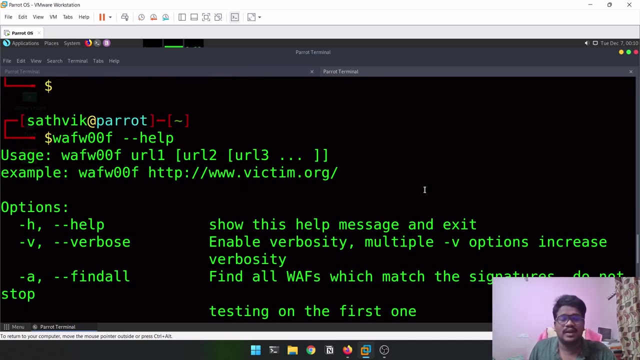 uh kali. you will have that by default. so let us look into the options. hyphen- hyphen help to the uh to view some options. like there are some many options out there like you can test for the whole uh, like, uh. like you can provide a file which consists of the urls, you can provide them and 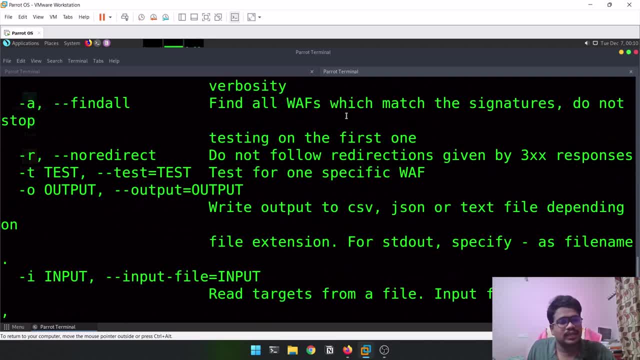 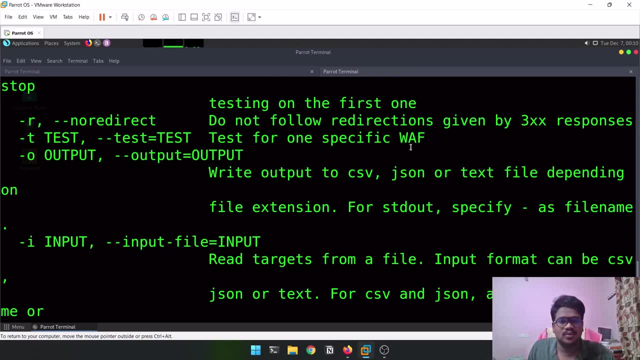 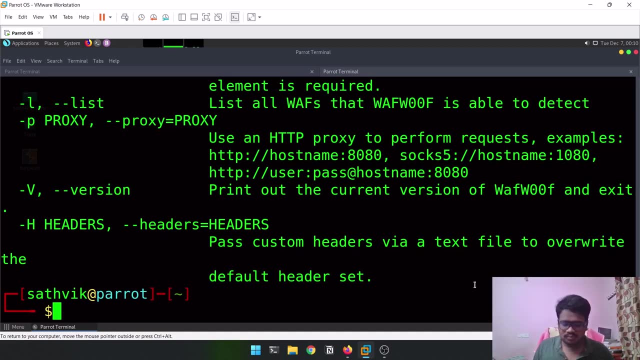 anything, everything goes, fine. okay, like you can make use of them. you can see some no redirect policies, like if there is a responses for three xss, so it doesn't follow. there are some kind of thing like that. you can provide a list, uh, to check for wafts and kind of thing. okay so. but 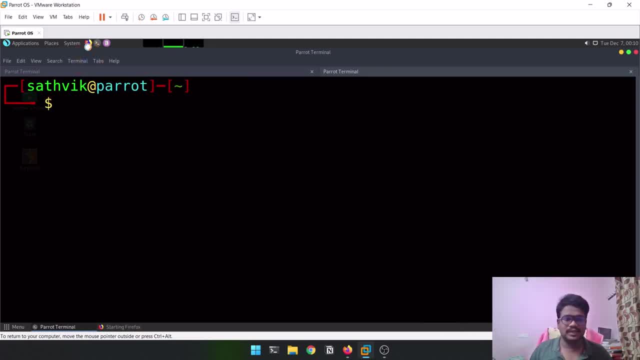 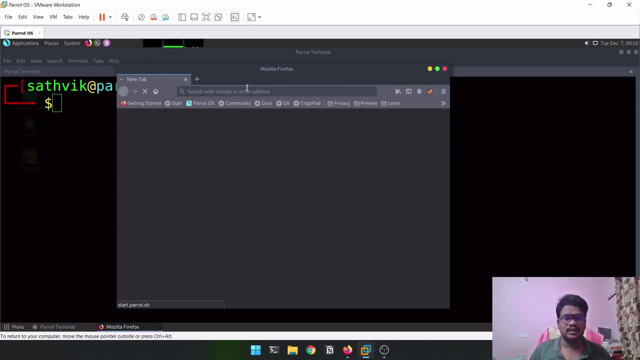 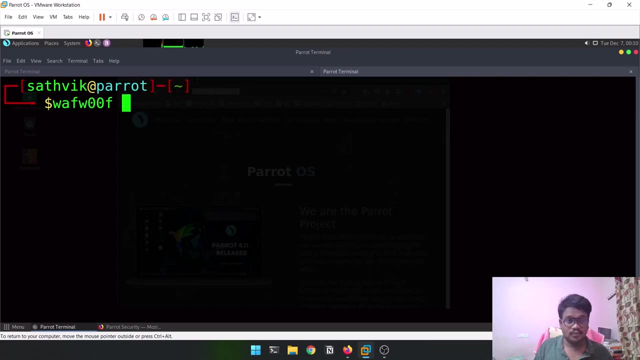 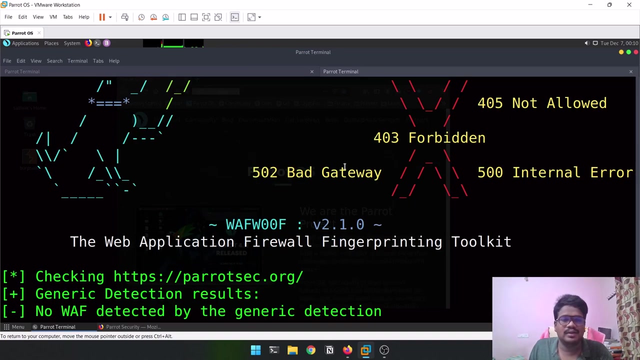 let me have a look here. so let me just have a look. so let me have a look. let me go to Weld. you have one problem. let me create one there. we have website, website. we actually have you know kind of a browser. uh, become online for me. 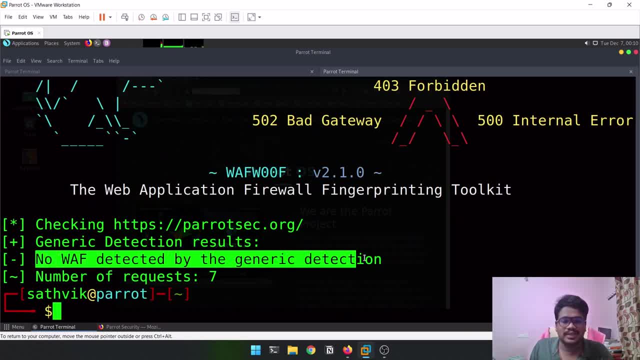 let me copy it and save it inside the website, inside the web site. okay, so now you can see that it is always a simple thing. so let me open a simple website. give us the work to just open a simple website like that. you can see there is no firewall detected by the generic detection. okay, so? 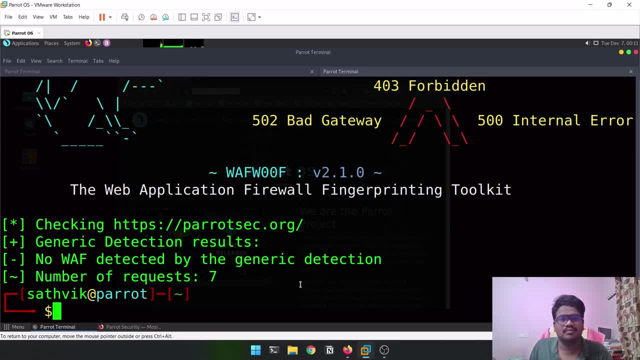 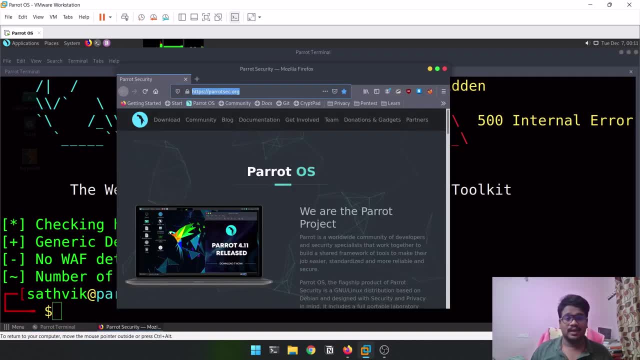 the requests are also few. like it sends some uh normal, like some limited amount of uh requests, and it is going to detect it. now i'm going to show you a website which have a what you call firewall used in for it. most of the time you might find a. there are some few firewalls and most 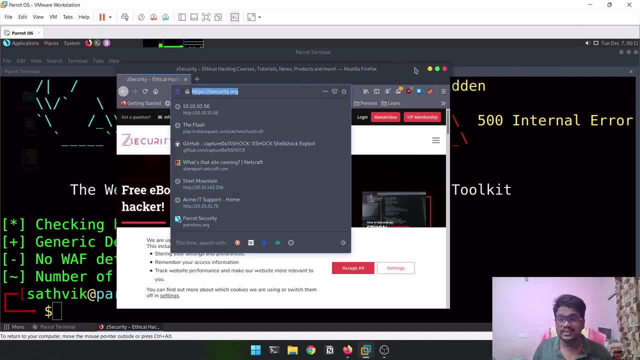 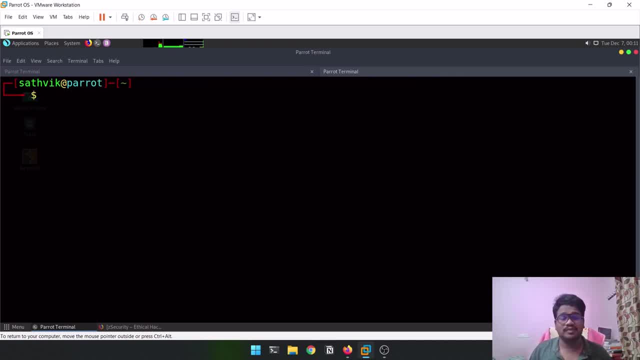 most popular one is uh, this particular thing called as cloudfare. it is most popular one and, like almost like most of the uh web application, fire web applications use that particular thing. so i'm going to uh do that. i'm going to test on jet security dot org. remember this is not. 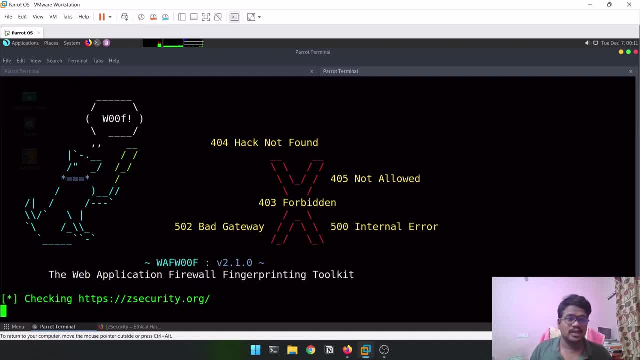 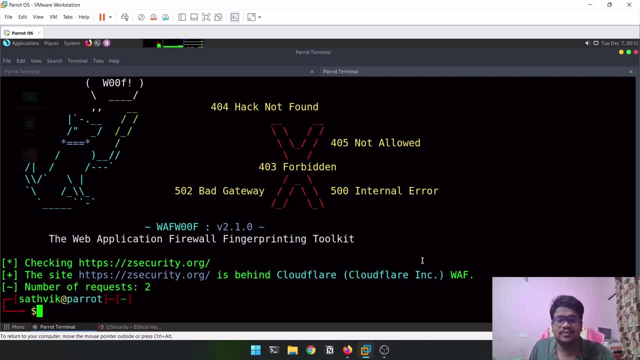 any harmful stuff, it is just information gathering. so let me hit enter so you can see that this particular site is behind cloudfare. so it is going to detect the web application firewall with their own something like, uh, with their own signature kind of stuff. okay, like they send some few, uh, what you call some. 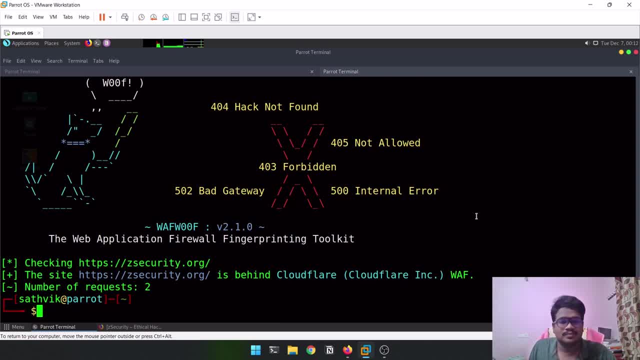 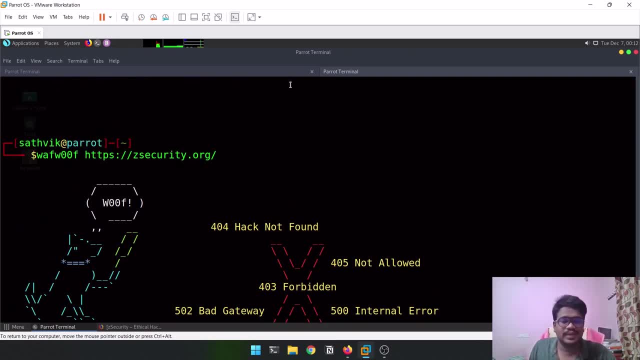 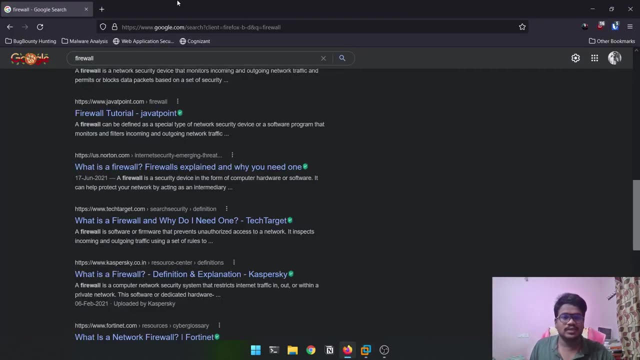 payloads and, based on those, it will try to detect it. so this is how you can make use of this particular tools like, uh, this nmap, as well as this wafoo, in order to detect this firewall. so once you get detected, like once you find, this is cloudfare. so you can see what you can simply do is like: 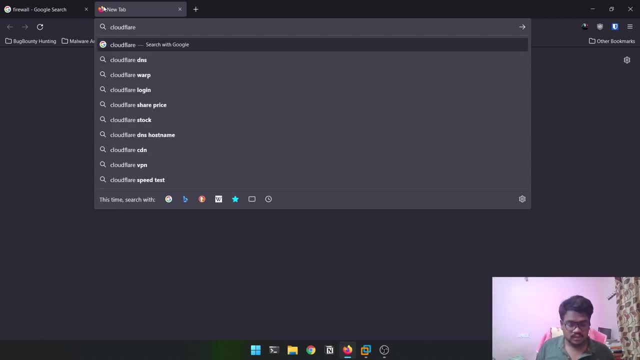 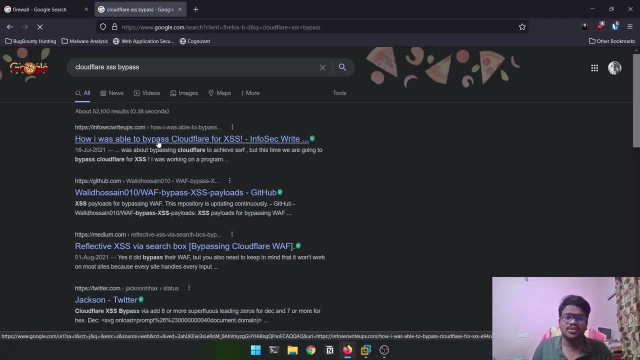 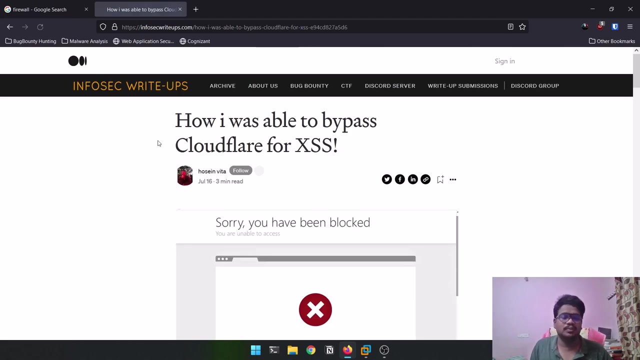 cloudfare, um, xss bypass. like you can simply go ahead and you can look for some resources. okay, like, most of the time, what happens is like, uh, you can't like, even though there is a possibility to run a simple javascript, it doesn't work. you need to do some modifications, like there are some few. 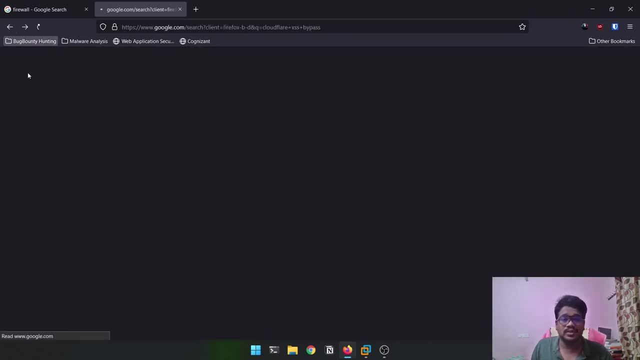 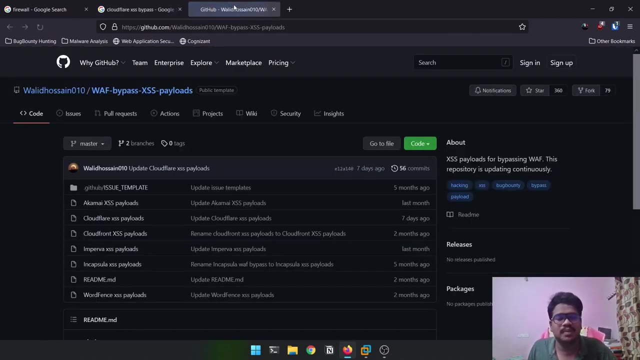 blocks out there and all you can check out them. also, there are few payloads, okay, like you can see. there are a few payloads as well, like i'm showing this for cross-site scripting, but you can make use of anything. okay, you can see cross-site scripting. this is what i'm showing you. 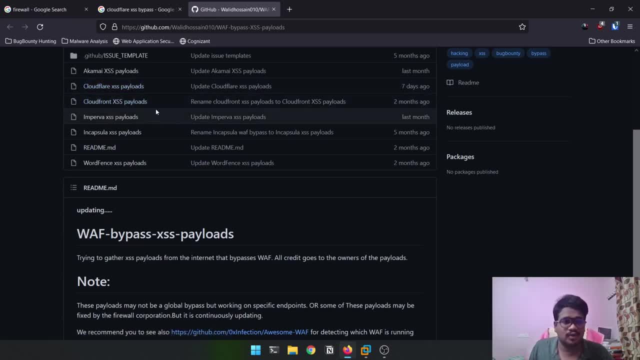 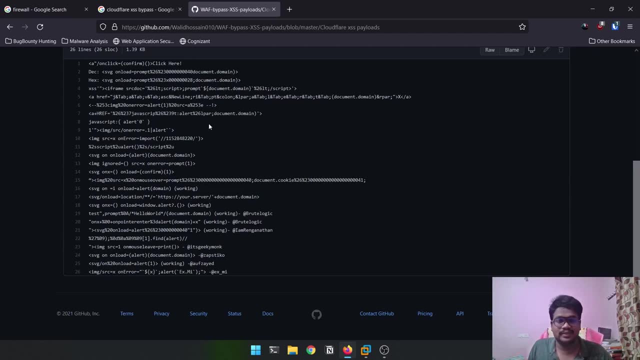 cloudfare, cloudfront- even those are some different kinds of firewalls. okay, so if you go to the xss payloads- like i'm not saying that these works all the time, but you need to put an eye on these things, okay, once you find there is a firewall, then it is always a better way to check out these. 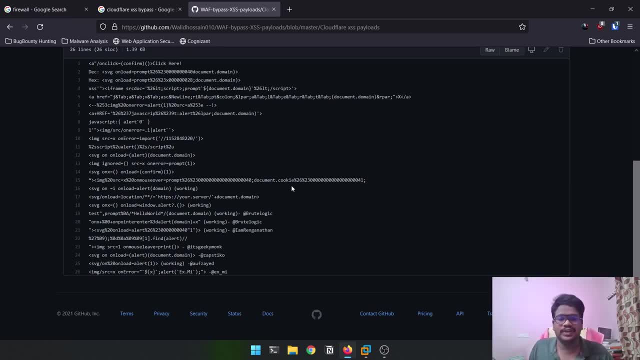 resources. so that is it, guys, for today's video, and i hope, uh, and i hope you found this video really helpful and uh, to summarize, in this video i had shown you a few tech, few techniques in order to detect the web application firewall, and if you like this video, make sure you like it and do share.